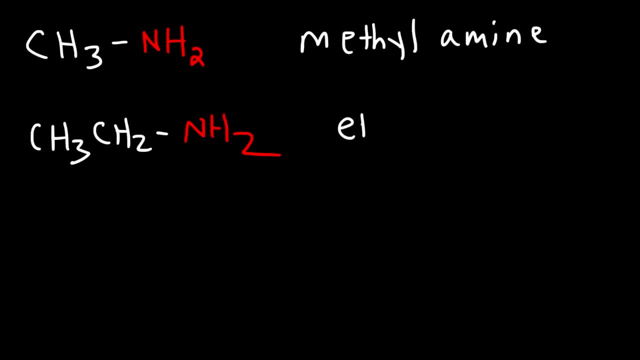 based on the previous example, you could see that this is called ethyl amine. Try this one. So what we have here is an isopropyl group attached to an amine, So this is going to be called isopropyl amine. 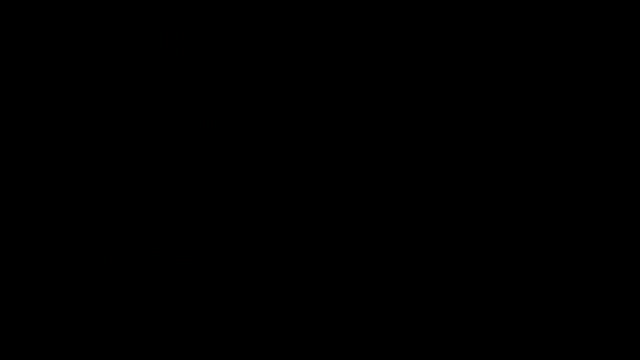 And it's wonderful. One word Now. let's work on some other examples. Here's another one that you could try. Go ahead and write the common name for that molecule and also for this one too. So go ahead and try those two examples. 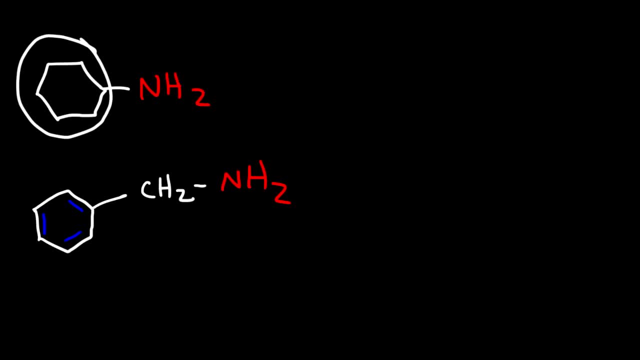 So we have a cyclohexane ring attached to an NH2 group, So this is going to be called cyclohexoamine. Now we have a phenyl ring, but with the CH2 it's now a benzyl group, So this is going to be called: 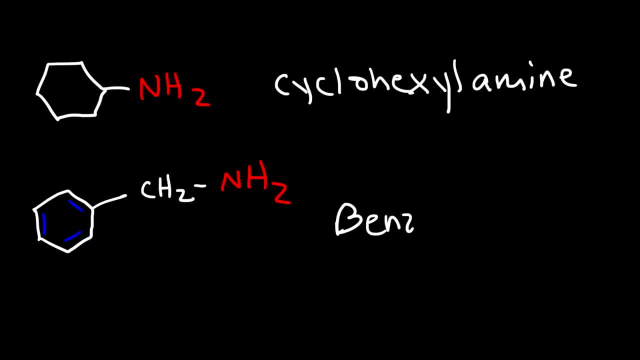 benzyl. This is freed from CH3 and this is now an amine. Try this example. Go ahead and name this particular molecule. What is the common name for this particular molecule? So, without the CH2 group, this is a phenyl ring. 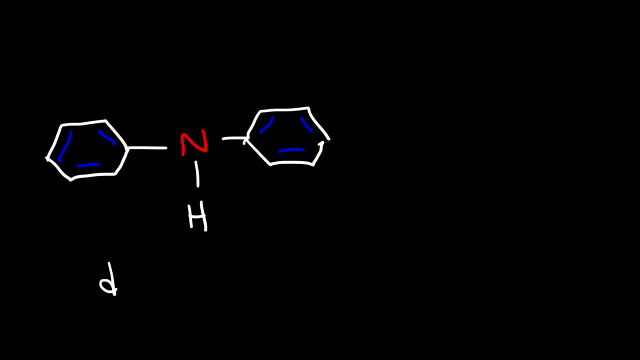 So we have two phenyl rings, And so it's going to be called diphenyl amine. Now let's move on to the next example. So let's say, attached to this nitrogen, we have a hydrogen and two methyl groups. How can we name this particular amine? 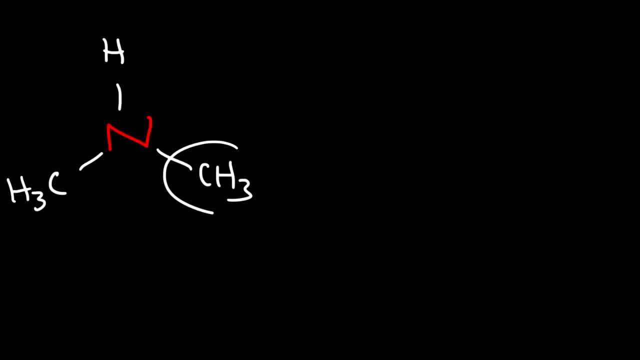 So, because we have two methyl groups attached to it, this is going to be called dimethyl amine. Now, what about this molecule? NCH2CH3 times 3.. Go ahead and name that molecule. Now we have three ethyl groups attached to the nitrogen atom. 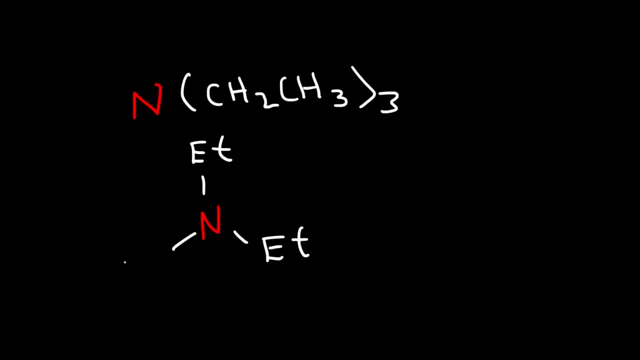 So I can write ET for short or you can literally write all the ethyl groups attached to it, And of course we know that there's a lone pair on the nitrogen atom, But to name it it's simply going to be triethyl amine, because there's three of them. 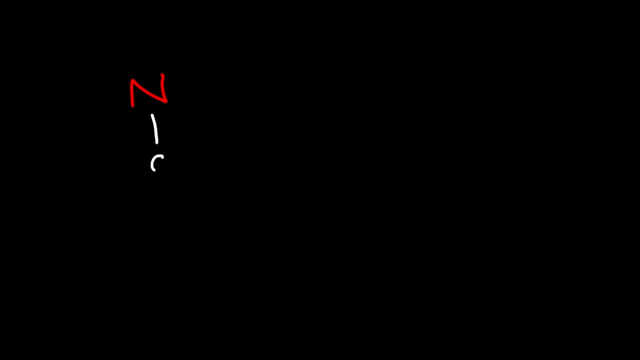 Now let's work on this example. So let's say we have an ethyl group, a methyl group, and another ethyl group attached to this nitrogen atom. What does the name of this particular mean? So, because we have two ethyl groups, that's going to be called diethyl. 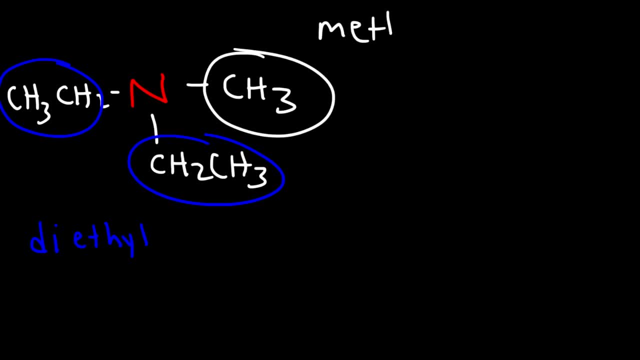 And we have one methyl group, so methyl, And then, because we have different substituents, we need to put it in alphabetical order, So we ignore the di part. E comes before M, So this is going to be called diethyl methyl amine. 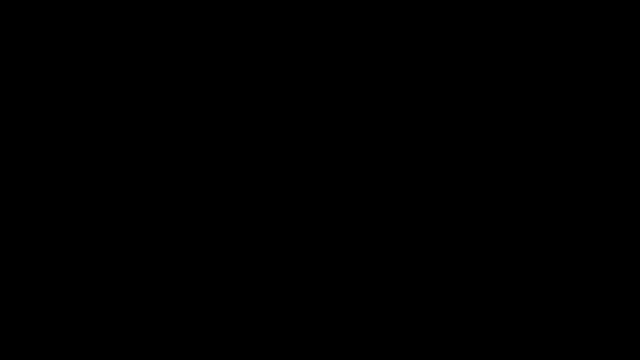 So that's the common name for it. Now let's consider one more example with common names of amines. E comes before M. Go ahead and name this particular amine. So on the left side we have a propyl group, on the right side an ethyl group and at the top a methyl group. 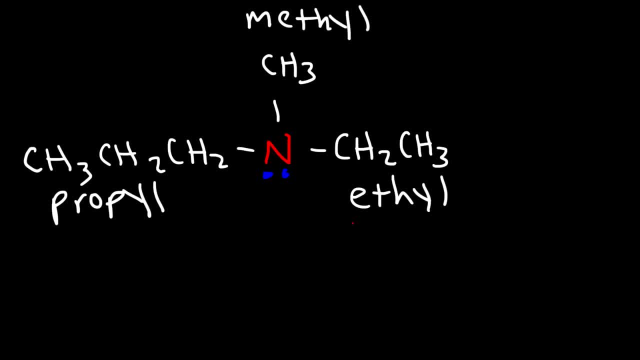 So how can we put this together? Well, we know that ethyl comes before methyl, E comes before M And M is before P in the alphabet. So, to put this all together, it's going to be ethyl methyl propyl amine. 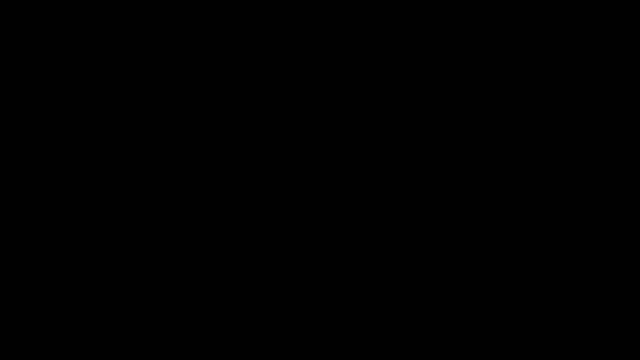 Now let's shift our focus to the IUPAC nomenclature of amines. So let's begin our discussion with this example. So the first thing we need to do is count the number of carbons in the longest chain. So there are three carbons. 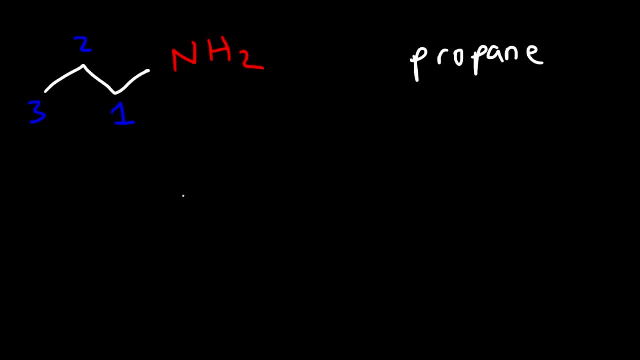 So we have propane Now. the functional group is an amine, So what we're going to do is we're going to drop off the E and replace it with amine. So this is propanamine. Now we need to talk about where the NH2 group is located. 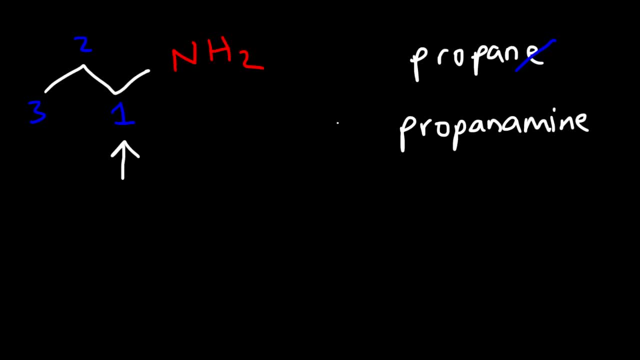 Okay, And, as we can see, it's located on carbon 1.. So this is 1-propanamine, And that's the answer for this example. Now let's try another example. Go ahead and name this particular amine. Feel free to pause the video. 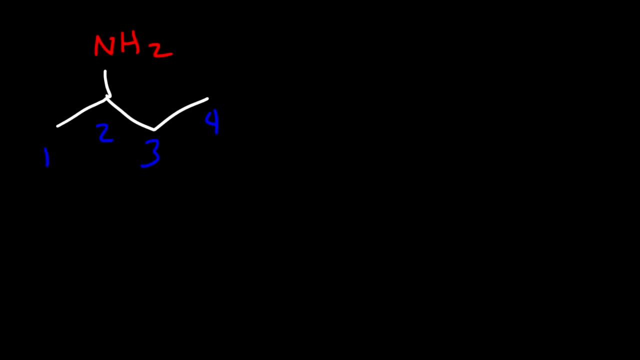 So let's begin by counting the longest chain, And so we have four carbons, which is associated with butane. Now let's try another example. So we're going to drop off the E, replace it with amine, So this is going to be butanamine. 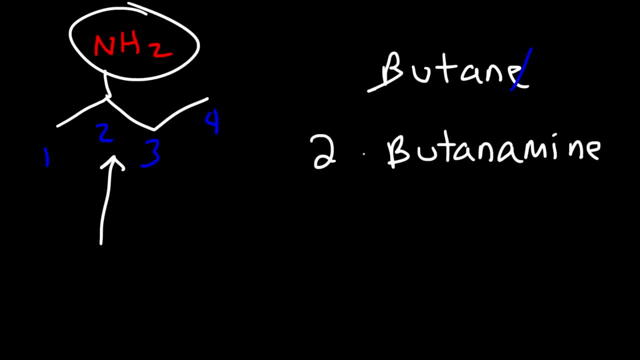 And the NH2 group is located at carbon 2.. So it's 2-butanamine. Now let's talk about our next example. So let's start with a molecule. Go ahead and name that molecule, Now which way should we count it? 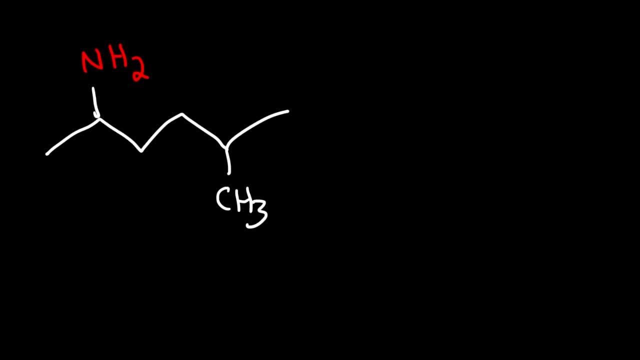 Should we count it from left to right or right to left? Now, the amino group has more priority than the methyl group, so therefore we want the amino group to have the lower number. So we're going to count it from left to right. 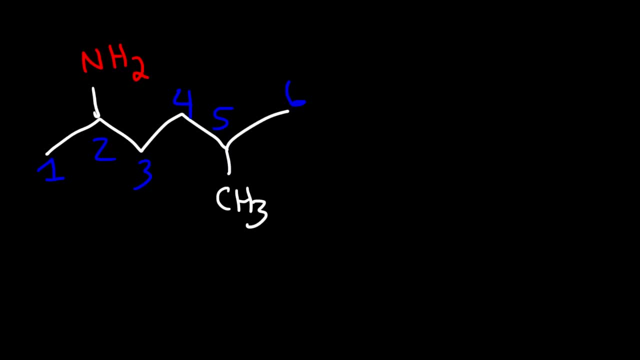 Either way we count it, the substituents will be 2 and 5, but we need to give this priority. So we have a hexane ring- I mean not a hexane ring, but a hexane chain- and we're going. 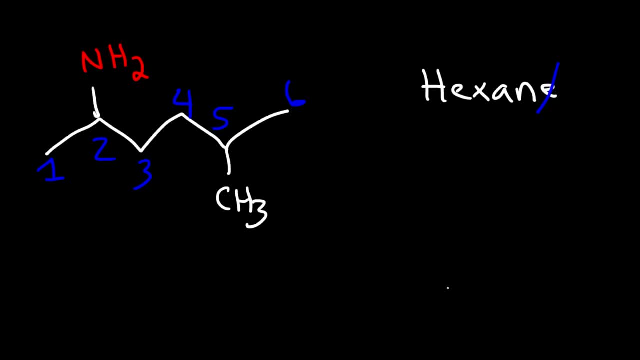 to drop off the E and replace it with amine. So this is going to be hexanamine. Now the amine is on carbon 2, so 2-hexanamine, and then we have a methyl on carbon 5.. 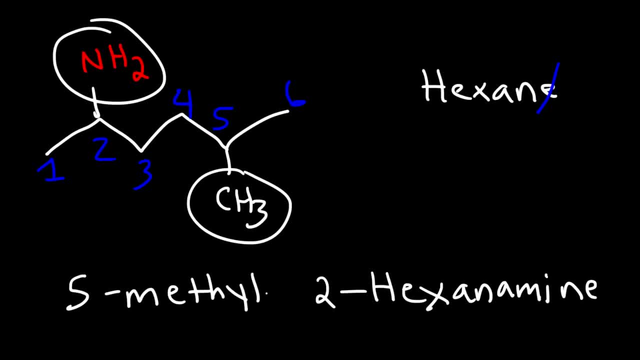 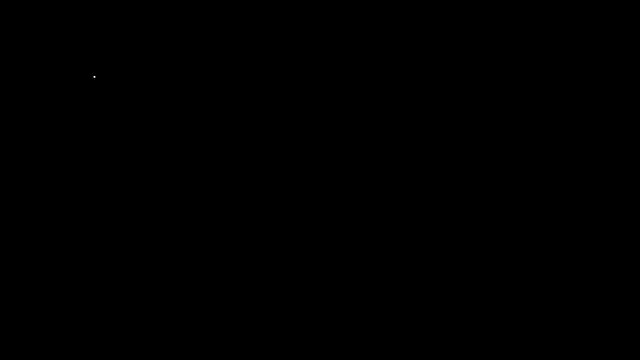 So this is going to be 5-methyl-2-hexanamine, And so this is the answer. Now what if we have, let's say, a nitrogen atom attached to a methyl group. at the same time, it's attached to a long carbon chain. 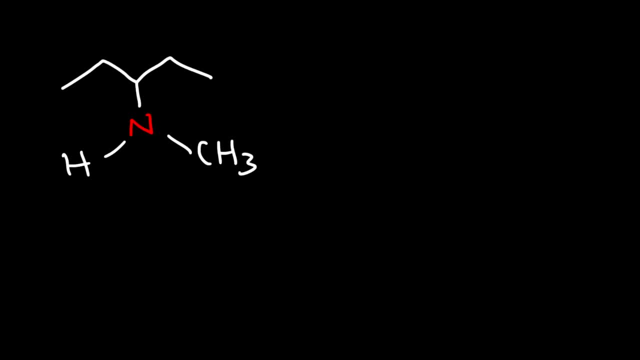 How can we name this particular amine? So we're going to follow the same example as we've been doing before. So we're going to count the number of carbons in the longest chain, So that's going to be pentane, but dropping off the E, it's going to be pentanamine. 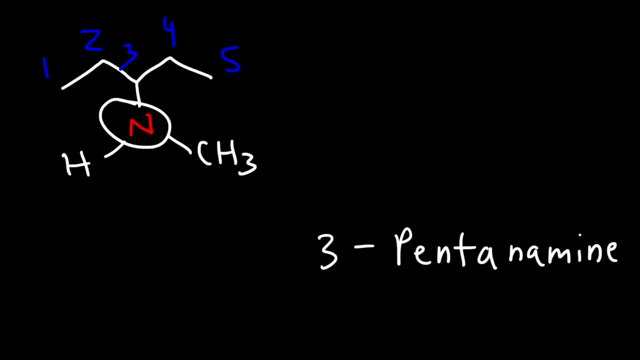 Now the nitrogen is on carbon 3, so it's 3-pentanamine. Now notice that we have a methyl group on the nitrogen. So what we're going to say is N the methyl, because the methyl is on the nitrogen, not 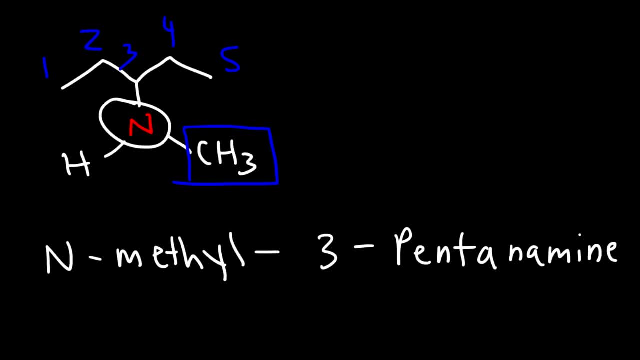 on the parent chain, dash 3-pentanamine. So, based on the last example, go ahead and try this problem. So this time the nitrogen is still attached to a long carbon chain, but we're going to attach a methyl group to it and an ethyl group to it. 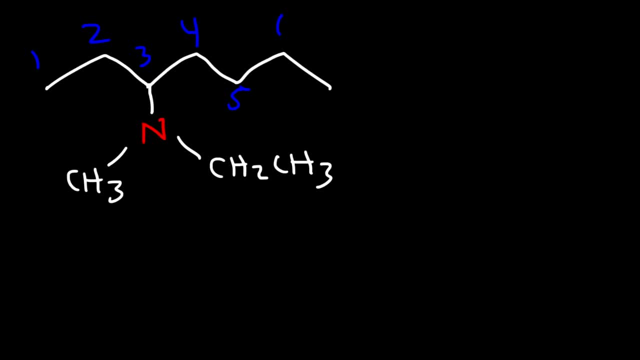 So let's begin by counting the number of carbon atoms in the longest chain. So we have a heptane chain. Instead of saying heptane, it's going to be pentane. So we're going to count the number of carbon atoms in the longest chain. 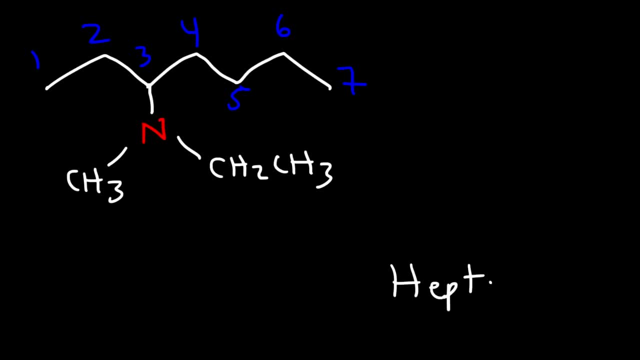 So we have a heptane chain. Instead of saying heptane, it's going to be heptanamine, And the nitrogen atom is on carbon 3 of the parent chain. So we have a methyl group and an ethyl group. 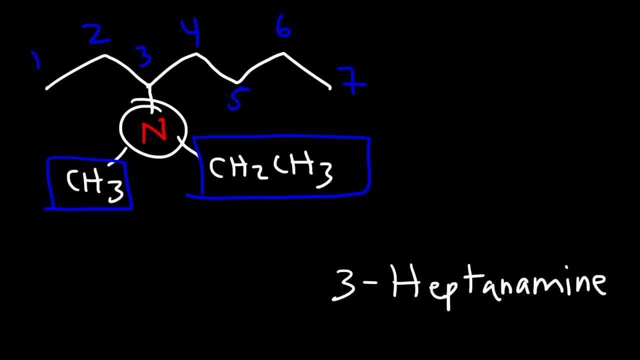 Now we need to put it in alphabetical order. so we're going to start with ethyl, So it's N-ethyl, because the ethyl is on the nitrogen atom, and then dash N-methyl, dash 3 heptanamine. 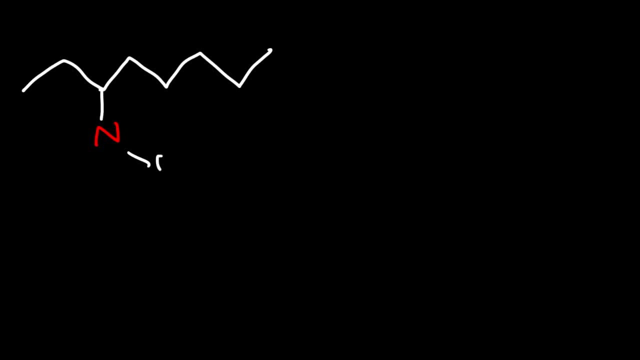 Go ahead and try this one. So this time we're going to have two methyl groups as opposed to a methyl and an ethyl group, So we have a total of eight carbon atoms. in the longest chain This is going to be octanamine. 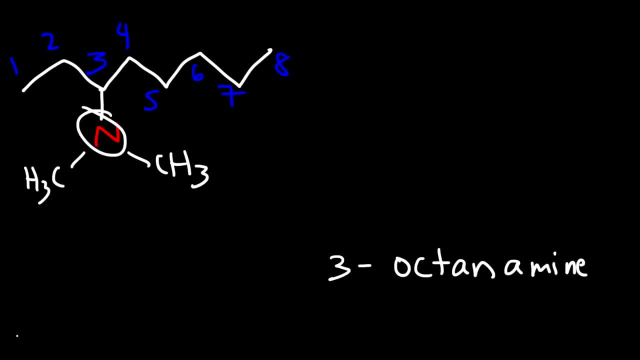 And the nitrogen atom is on carbon 3,, so 3-octanamine, And, as we can see, we have two methyl groups. So this is going to be NN-dimethyl because we have two of them: dash 3-octanamine or 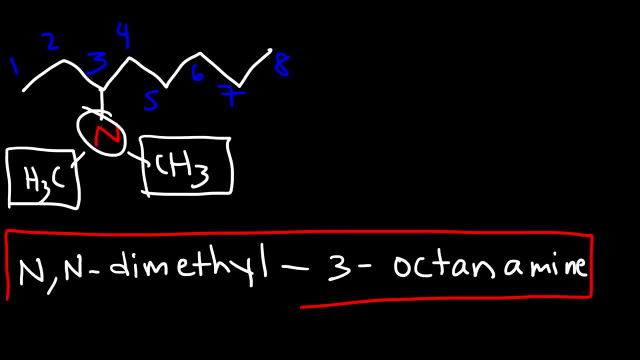 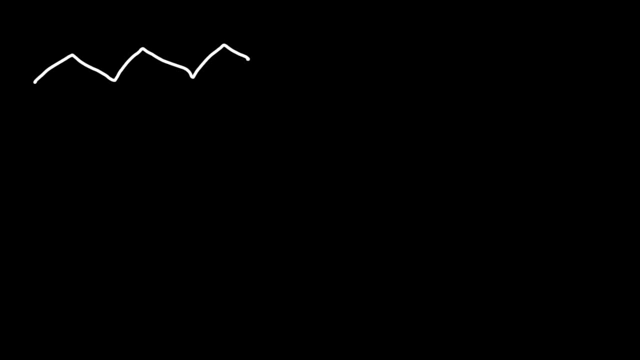 3-octanamine. That's it Now. let's work on this example. So let's put a halogen on the chain, Go ahead and name this particular molecule, So we know the nitrogen is going to have priority. This has to be number one. 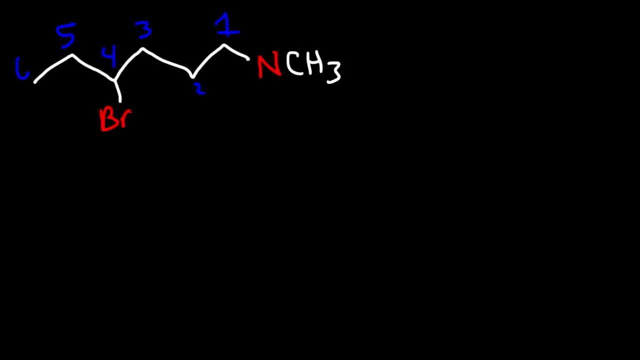 So this is carbon 2,, 3,, 4,, 5, and 6.. So we have hexane. Let's replace the E with amine. Now the nitrogen atom is on carbon 1, so this is 1-hexanamine. 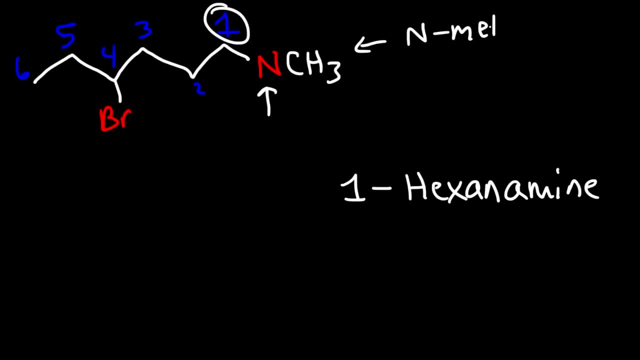 Now we have an N-methyl group, a methyl group attached to the nitrogen, and we have a bromo group And this is attached to carbon 4.. So we need to put it in alphabetical order: B comes to 4M. 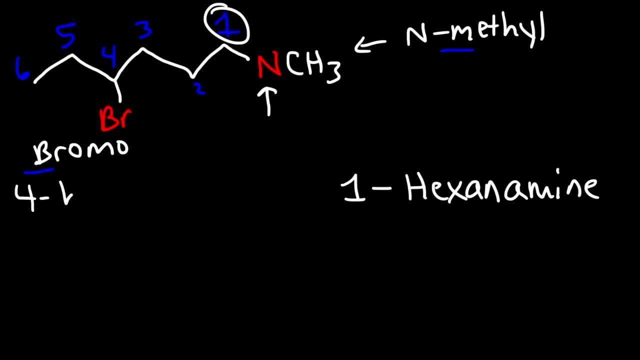 So therefore, this is going to be 4-bromo dash, N-methyl dash, 1-hexanamine. Now what if we have two functional groups, Let's say An NH2 group and an OH group? Which group will have priority? 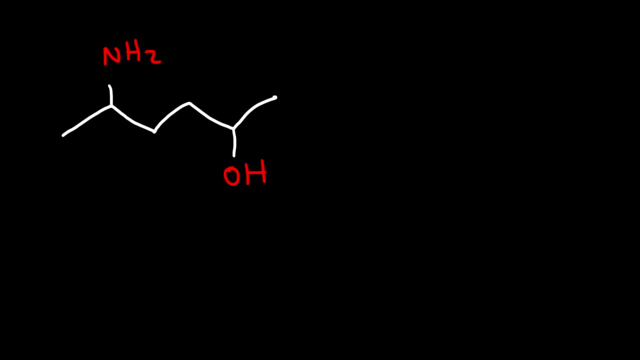 It turns out that the alcohol group has more priority than the NH2 group, And so the NH2 group is going to be treated as a substituent. In this case, it's going to be called amino as a substituent. So because the OH has more priority, we're going to give it the lower number. 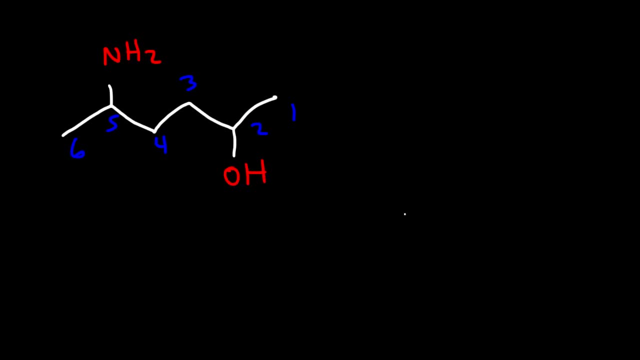 So instead of saying hexane as the parent name, it's going to be hexanol, because we have an alcohol And the alcohol is on carbon 2. And the NH2 group is on carbon 5. So it's 5-amino-2-hexanol. 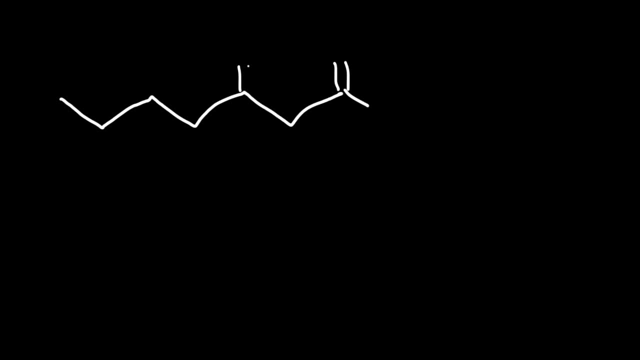 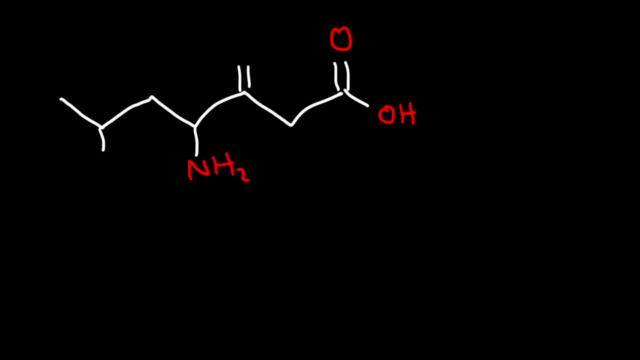 We have a molecule, We have a molecule, We have a molecule. So let's say we have a NH2 group, A carboxylic acid, An ether And also a ketone. So how can we name this molecule? Well, first we need to determine which functional group has the highest priority. 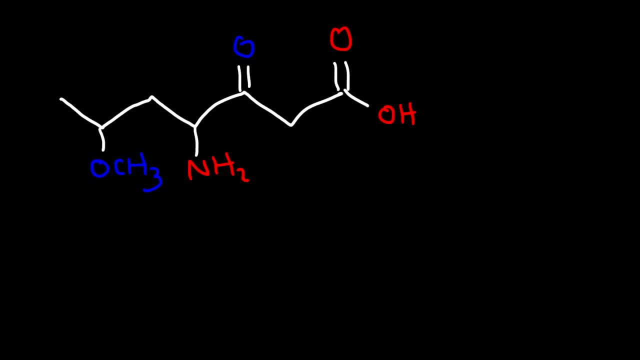 And out of all of these it's always going to be the carboxylic acid, always at the end, so automatically it's going to be assigned a number one. so we have a seven carbon chain which is heptane, but because we have a carbosilic, 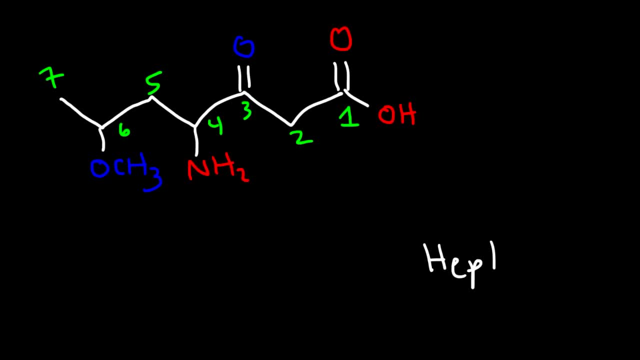 acid. it's going to be heptanoic acid and we don't need to say one heptanoic acid because it's automatically on carbon one. the carbosilic acid cannot be on carbon two, three or four. it has to be at the end. so now we have an oxo group. that's a 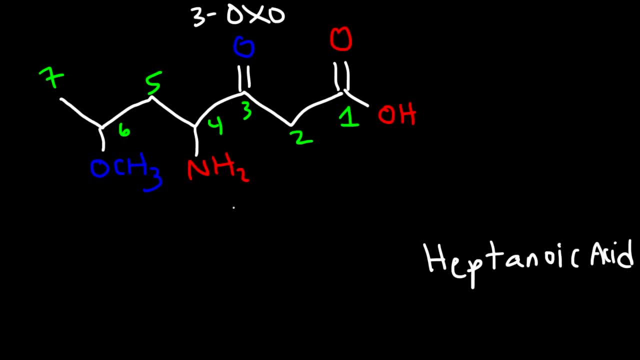 ketone. as a substitute, we have an amino group on carbon four and this is called methoxy, and so that's on carbon six. so we need to put it in alphabetical order, so the amino group comes first and then M is before O, So it's going to be 4-amino-6-methoxy-3-oxo-heptanoic acid. 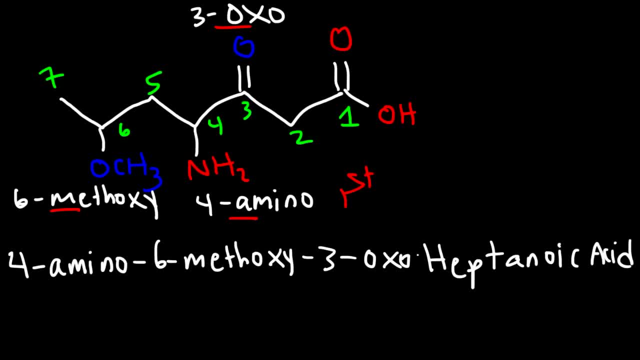 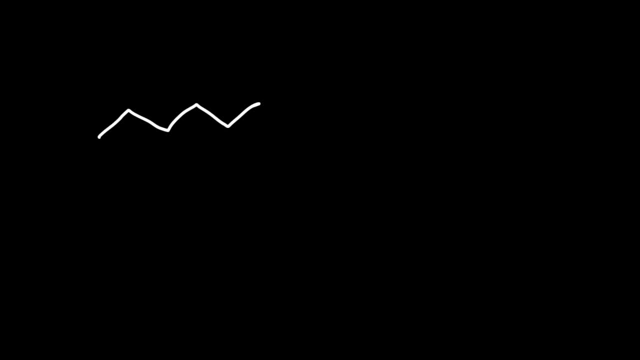 So that's how we can name this particular molecule. Now let's move on to our next example. So what if we have two NH2 groups attached to a chain? In this case, we have a 4-carbon chain, so that's butane. 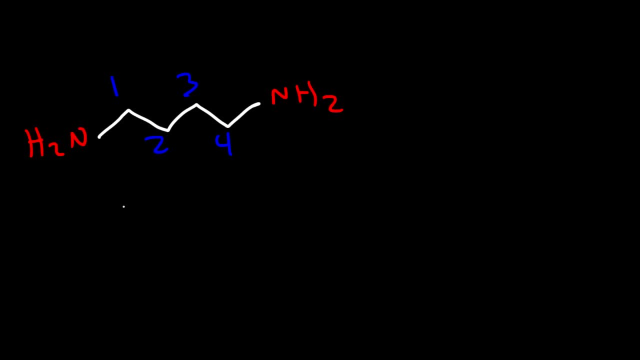 How can we name this particular amine? So we have an amine on carbon 1 and on carbon 4.. So it's going to be called 1,4-butane And di-amine. So this time we don't drop the E, because we have a consonant here. 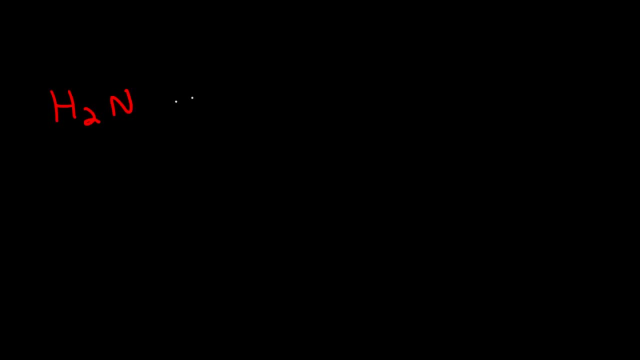 Let's try another similar example. Go ahead and name this particular molecule. So this is carbon 1,2,3,4,5,6.. We can count it in either direction, because it will give us the same name. So this is going to be 1,6-hexane-di-amine. 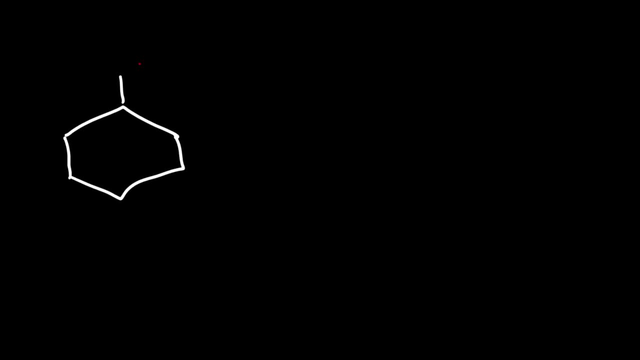 Now, this is going to be the last example, So I figured we should do one example with a cyclohexane ring. Go ahead and try this one. So, since we have a cyclohexane ring, instead of saying cyclohexane it's going to be cyclohexanamine. 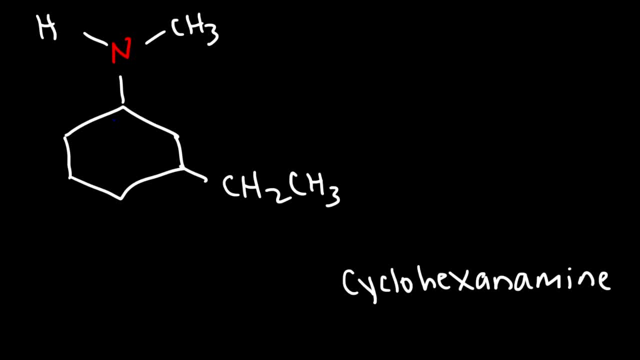 And the nitrogen has more priority than the ethyl group. so automatically this is carbon 1.. So we don't have to say 1-cyclohexanamine Now we do have a methyl on the nitrogen, so that's an N-methyl group. 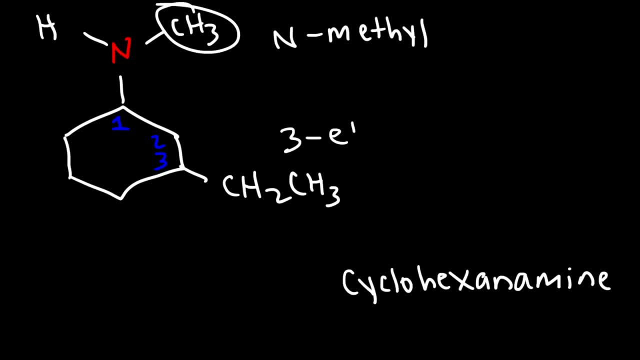 And we have an ethyl on 3, so 3-ethyl And E comes before M. So, putting it together, this is going to be 3-ethyl-N-methyl-cyclohexanamine, And so that's it for this video.